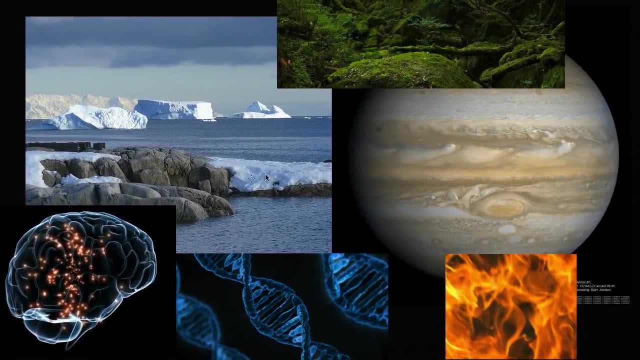 and it doesn't even have to be our planet, it could be the universe around us. you see all of these different substances that seem to be different in certain ways. You see things like fire and rock and water, even in the planets, you know. 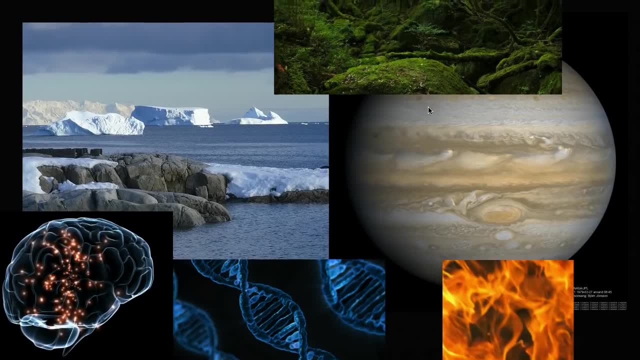 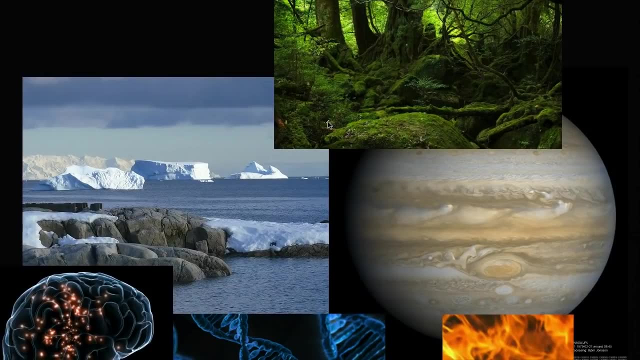 you see meteorological patterns In life. you see all of this complexity and all of these different things And it looks like there's just an infinite spectrum of differentness out there, of different substances, even things like our human brain, the complexity and the electrochemical interactions. 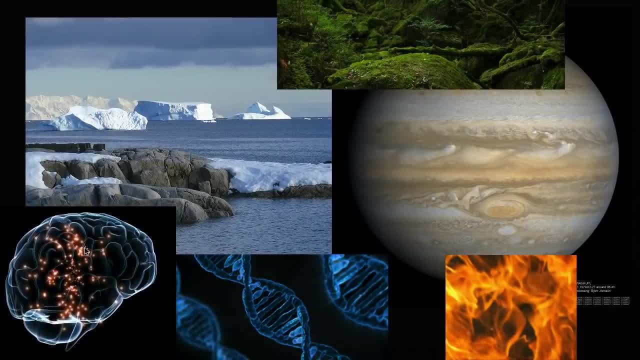 And you could imagine as a species. this is kind of overwhelming. How do you make sense of all of this? And it was not an easy path, But over thousands of years we did start to make sense of it And why it's very lucky for all of us to be born. 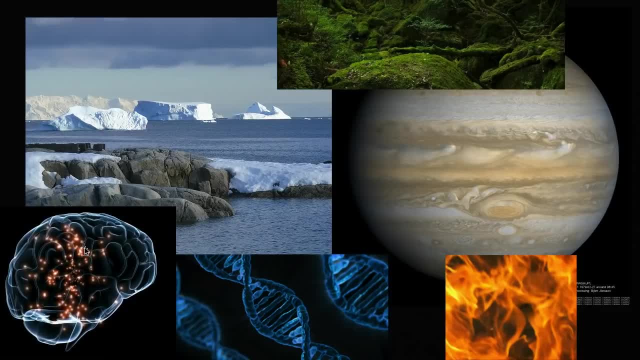 when we are now, or to be around when we are now to be able to learn chemistry. where we are now is that we get the answer, And it's a partial answer, which is also exciting because we don't want the full answer. 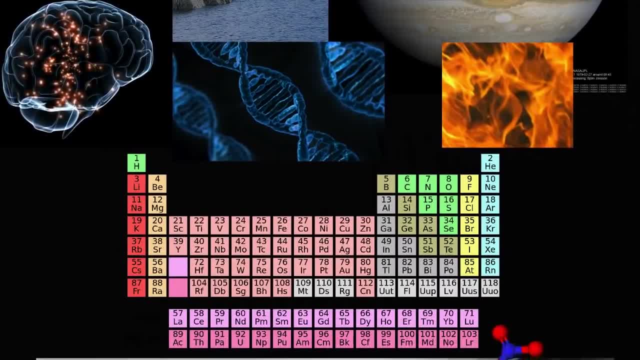 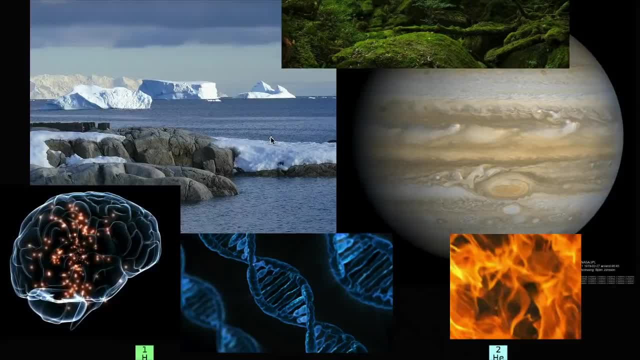 But it's a partial answer that takes us a long way. We realize that the periodic table of elements, that all of this complexity that we're seeing before, that at the end of the day, things are made of basic building blocks. You can imagine the Legos that really make up everything. 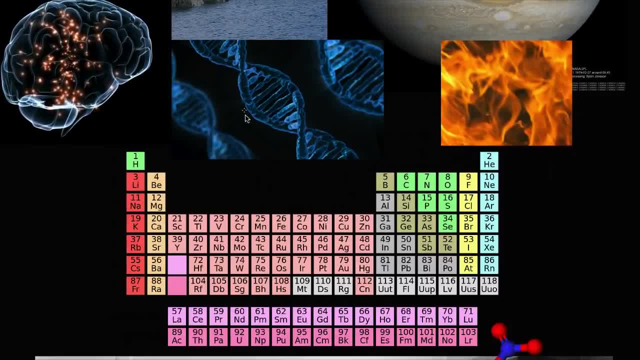 And there aren't an infinite number of Legos. There's actually a finite number, And we're discovering more all of the time. Well, not all of the time. Now new elements are not discovered that frequently, But there's a few of these elements. 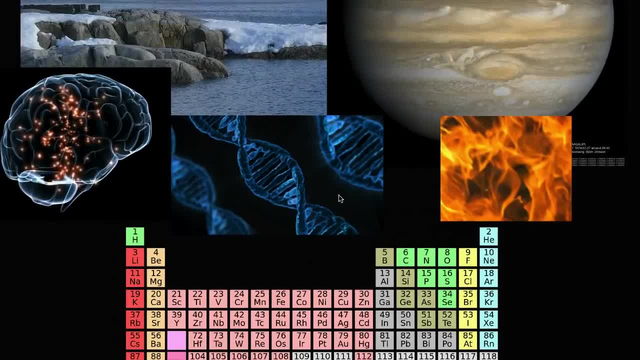 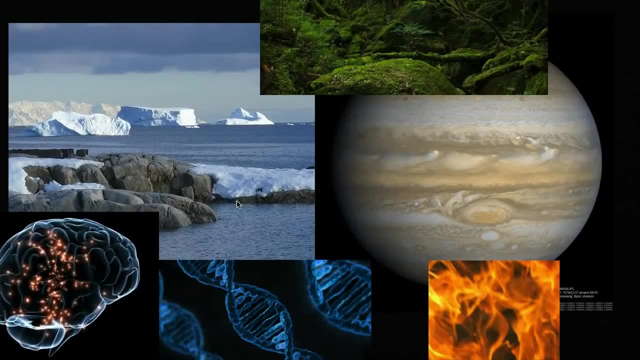 that are disproportionately showing up in a lot of what we see here, these things that seem so different. Well, a lot of this is different compositions of elements like carbon and oxygen and hydrogen, And even the elements themselves are made of things like protons and electrons and neutrons. 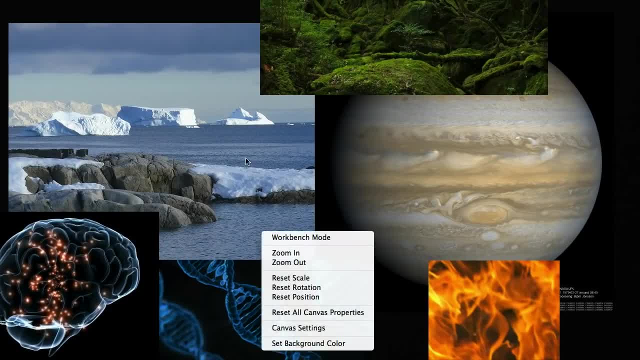 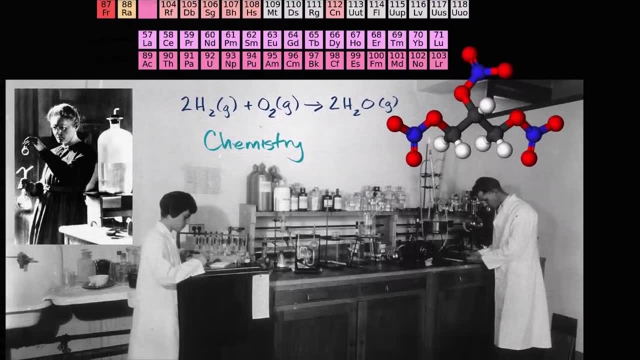 that are just rearranged in different ways to give us these elements that have all of these, that have all of these different properties. So when you think about chemistry, yes, it might have. it might visually look something like this: These are obviously much older pictures. 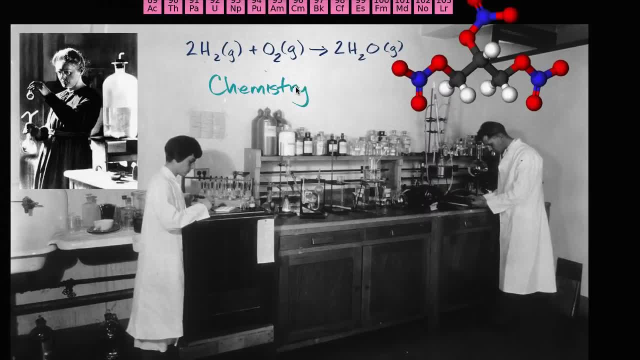 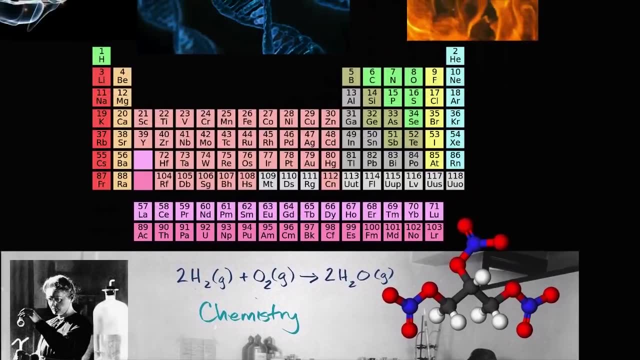 But at its essence it's: how do we create models and understand the models that describe a lot of the complexity in the universe around us And, just to put chemistry in, I guess you could say in context with some of the other sciences. 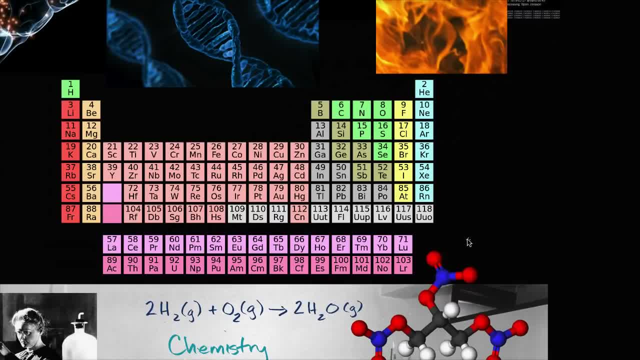 many people would say, at the purest level you would have mathematics, That math. you're studying ideas which could even be independent. you're seeing logical ideas that could be even independent of anything that you've ever observed or experienced. And a lot of folks that say 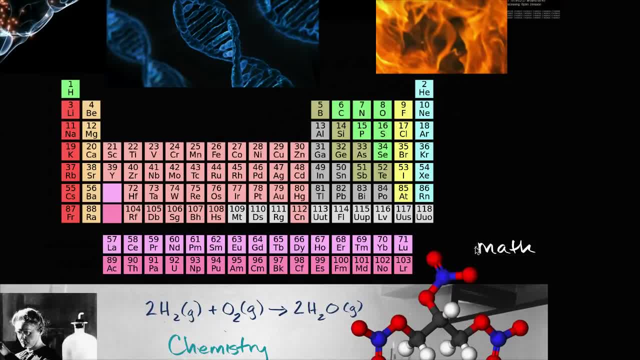 if we ever communicate with another intelligent species that could be completely different than us, math might be that common language, Because even if we perceive the world differently and think differently, in certain ways math might be that common language. Then, on top of math, we start to say: 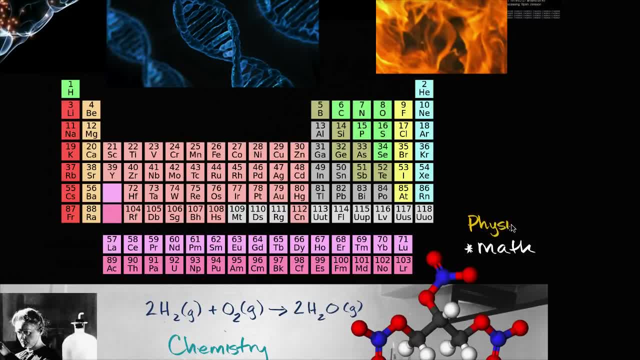 well, how is our reality actually structured At the most basic level? what are the constituents of matter and what are the mathematical properties that describe how they react together And then or interact with each other, And then you go one level. 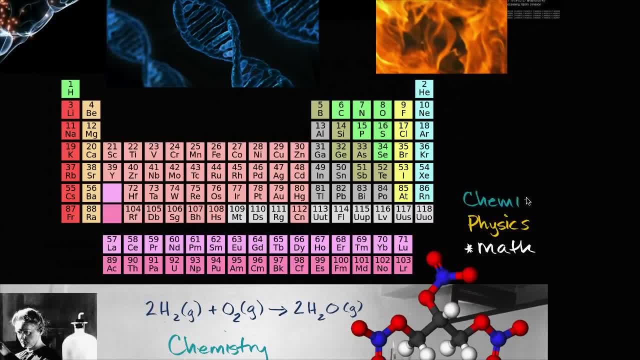 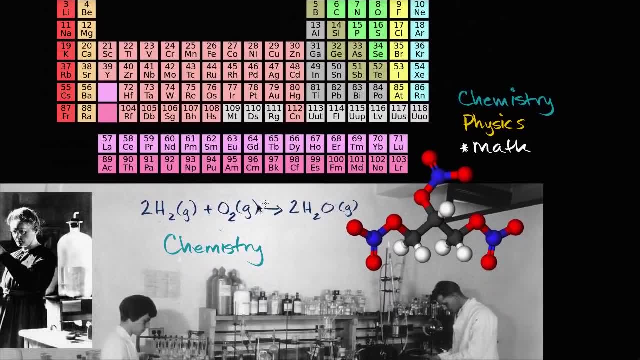 above that you get to the topic of this video, which is chemistry, which is really, which is very closely related to physics, When we talk about these chemical equations and we create these molecular structures, the interactions between these atoms, these are quantum mechanical interactions. 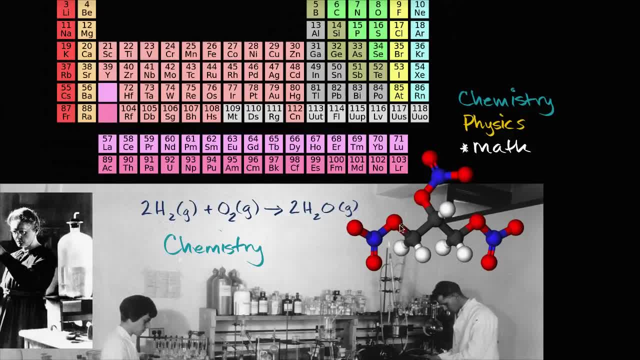 that we are, which we do not fully understand at the deepest level yet, But with chemistry we can start to make use of the math and the physics to start to think about how all of these different building blocks can interact to explain all sorts of different phenomena. 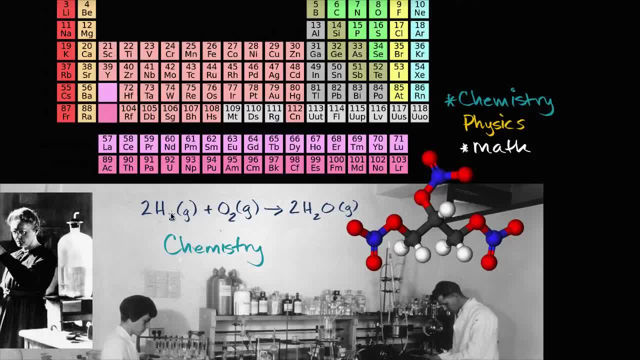 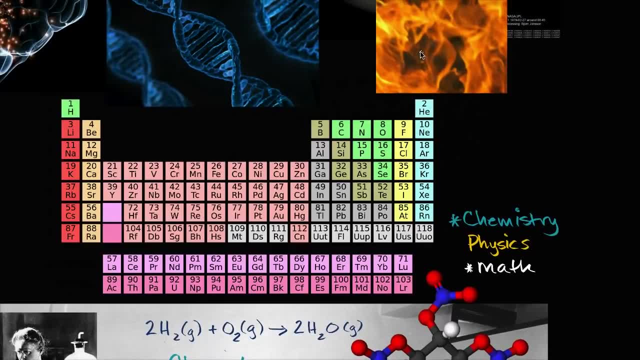 What we, this chemical equation you see right here. this is combustion, This is hydrogen combusting with oxygen to produce a lot of energy. To produce energy. and when we imagine combustion, we think of fire. But what even is fire at its most fundamental level? 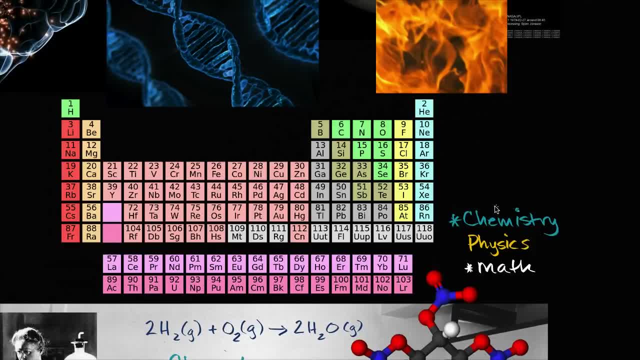 How do we get, why do we perceive this thing here? And chemistry is super important because on top of that we build biology And, as you'll see, as you study all of these things, there's points where these things start to bleed together. 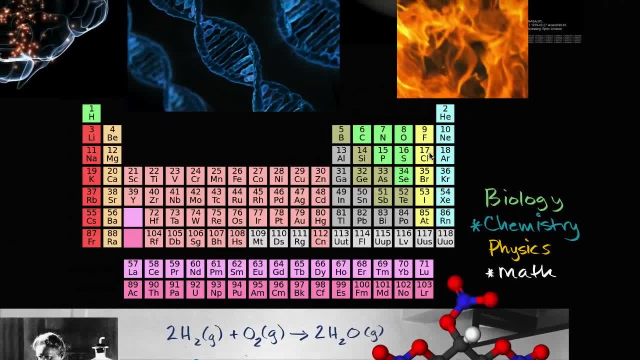 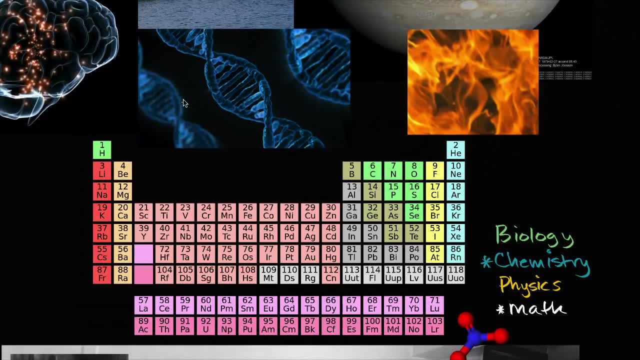 But the biology in, say, a human being, or really in any species, it's based on molecular interactions, interactions between molecules, between atoms, which, at the end of the day, is all about chemistry As I speak- the only reason why I'm able to speak- 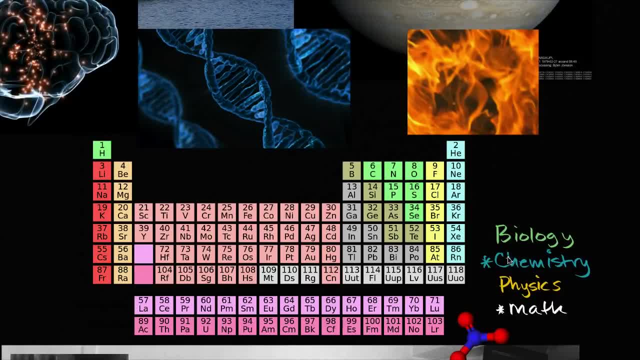 is because of really hard to imagine a number of chemical interactions happening in the atmosphere. What's happening in me right now? to create this soundness, to create this thing that thinks it exists, that wants to make a video about how awesome and amazing chemistry is. 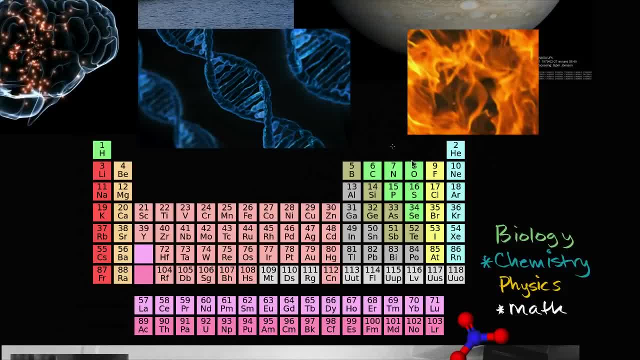 And then from biology you can build out on all of everything else, Scientists like psychology and economics- which of course these things also will leverage math and other things. But this gives you kind of a sense of how we build up and how we explain the reality around us. 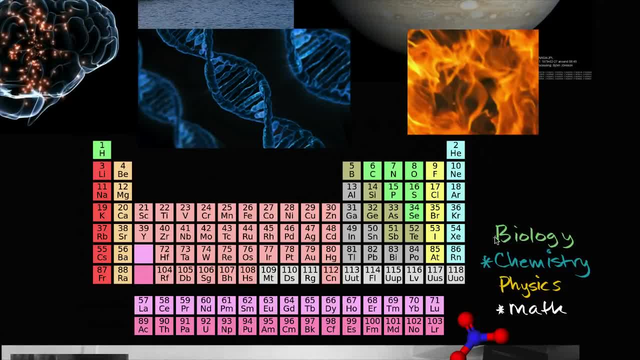 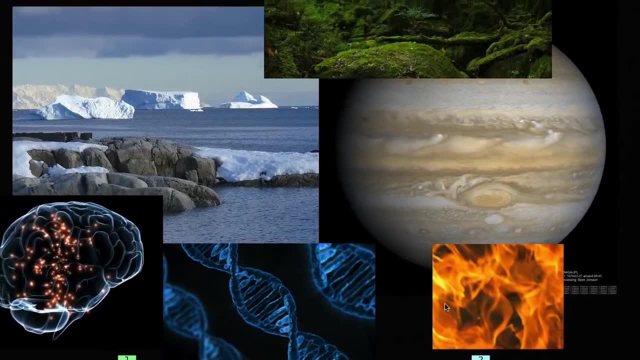 And not one of these is more important than the other. These are all studying incredibly fascinating things that, as human beings first became thoughtful about their environment, said: gee, why are we here? What is this place? Why do we exist? How do we exist? 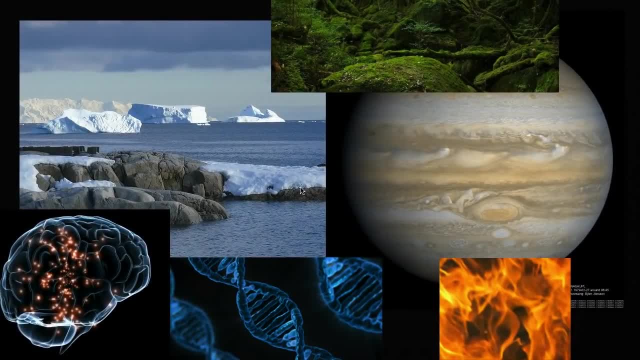 And chemistry builds models for us to understand interactions at a scale and a speed that we can't directly observe, but nonetheless we can start to make predictions. So that's what's really cool about this. When you study chemistry, you should not view this as some type of a chore. 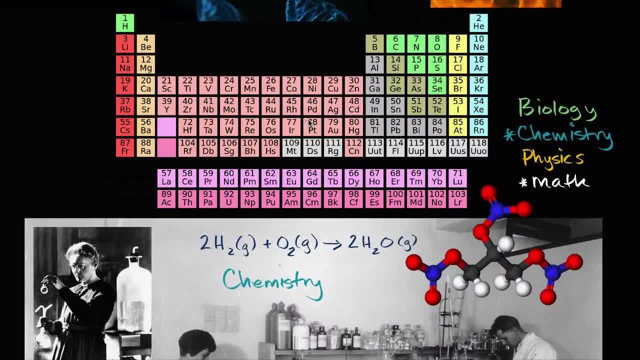 that the school system is forcing you through You are getting. there are people who would have done anything 100 years ago to get the answers that are in your chemistry book today, or that you could learn from your chemistry teacher, or that you could learn from a Khan Academy video. 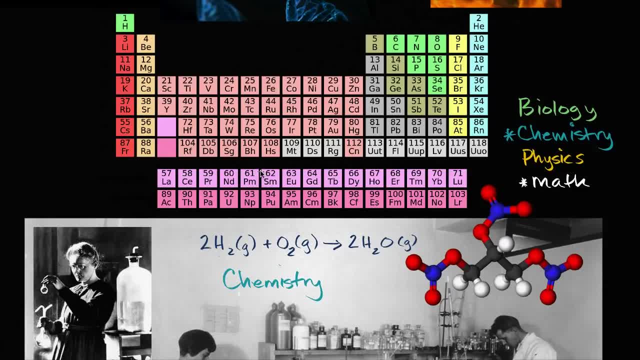 There are people in the world, in the past and today, who do anything to be able to understand deeply what this is. They consider it a privilege to be able to learn at this level And then to think about where this could go, because none of these fields are complete. 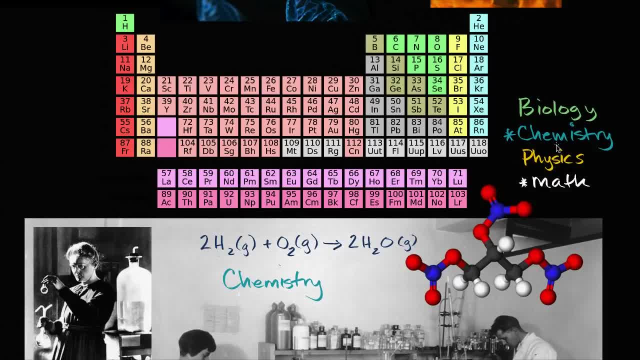 We have very partial knowledge of all of these fields. Arguably there's an infinite more that we can learn relative to what we know, But what's exciting is that we have such a strong start. We're starting to make sense of it, to really describe everything in our reality.